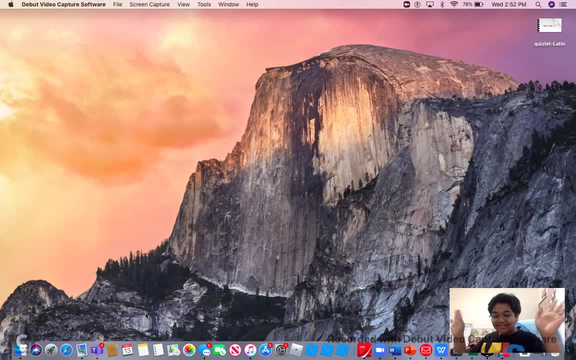 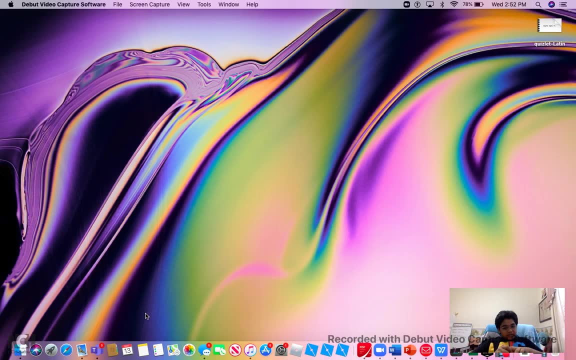 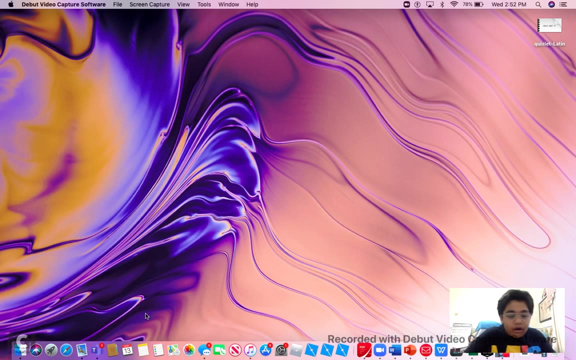 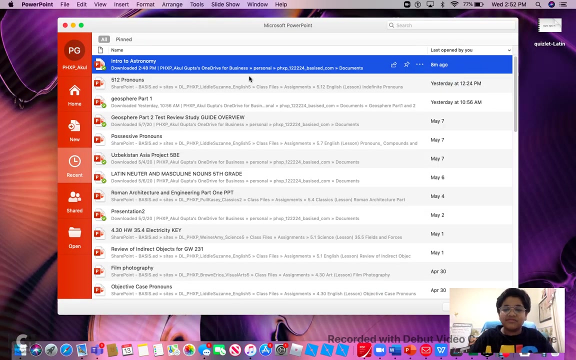 hey guys, how's it going? welcome back. so today we're gonna be continuing on with our astronomy and today we're gonna learn about galaxies and planetary systems. so let's get on to this PowerPoint. it's pretty small, but you know it's pretty good, it's okay, it's pretty good. so yesterday, you guys know, we did the. 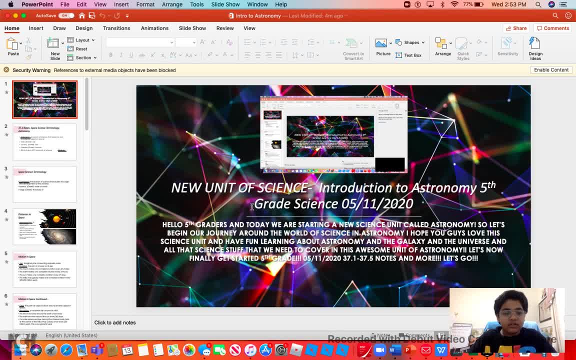 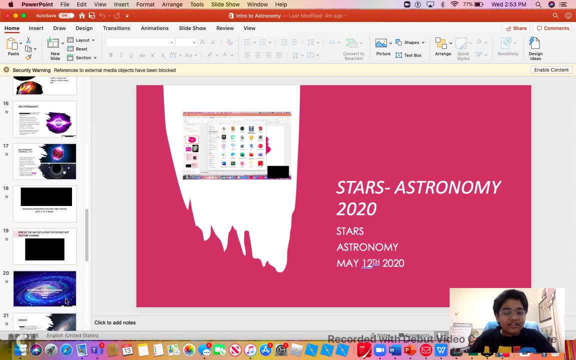 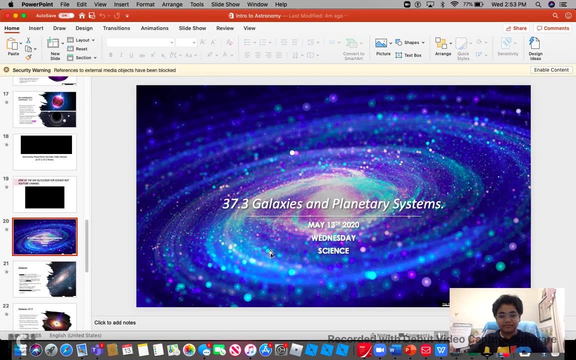 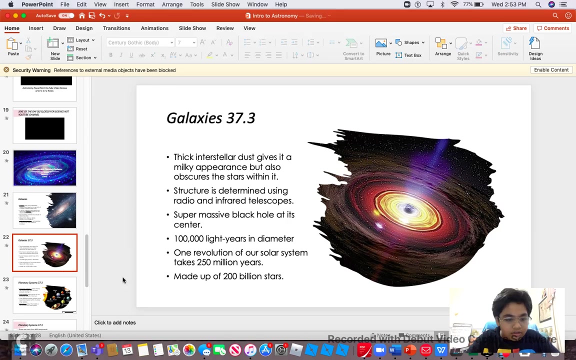 unit of science. we did space science, terminology, and then we did stars, and today we're gonna learn about galaxies and planetary systems. so let's get started. just give me just like a few more minutes before we get started. I have to do a few things here. I'm gonna get rid of a few things here. you know cuz I put. 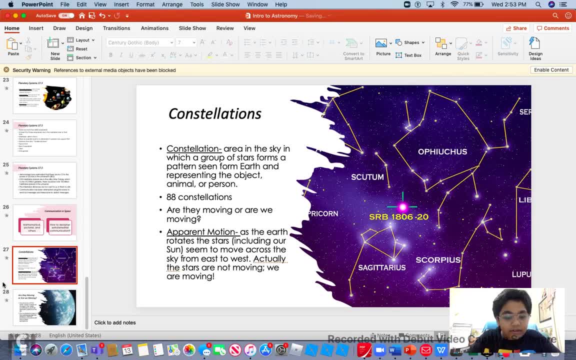 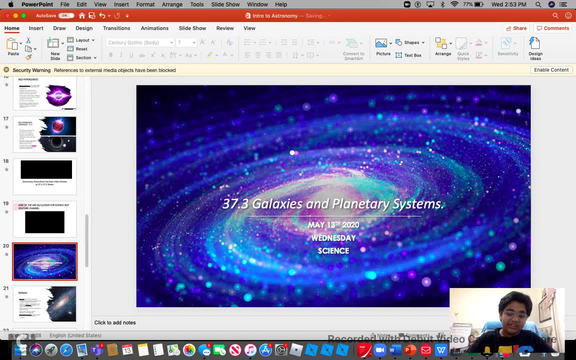 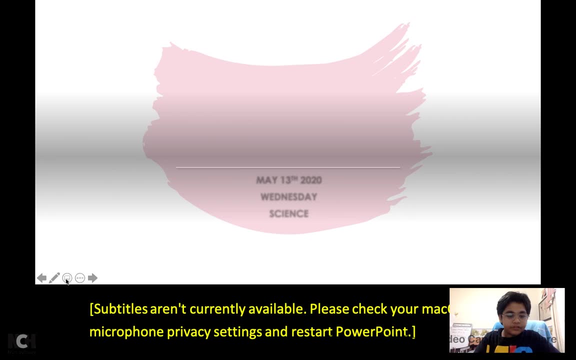 pictures, pictures has those things that I need, that you need to get rid of. and, yeah, it's okay, there's only eight slides, so let's just get on to it, okay, everybody? so so today we're gonna be talking about galaxies 37.3, which is today, Wednesday. 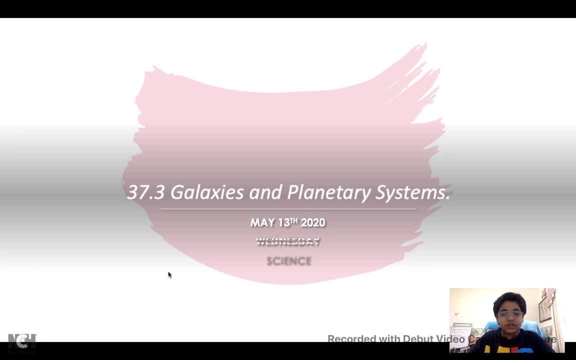 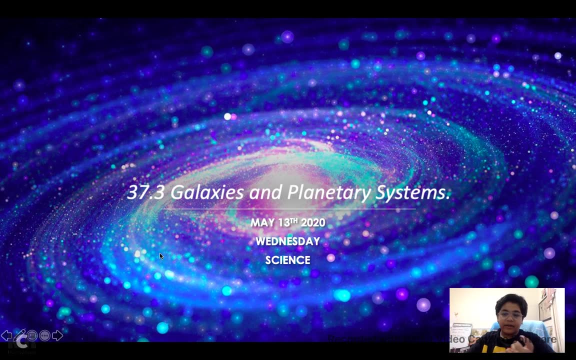 and planetary systems. so it's May 13, 2020 to Wednesday, science. so this is what a galaxy looks like: there's spiral, a ballistic, a ballistic and one more, which I forgot. but that's how a galaxy. okay, that's a spiral. let's move on to our 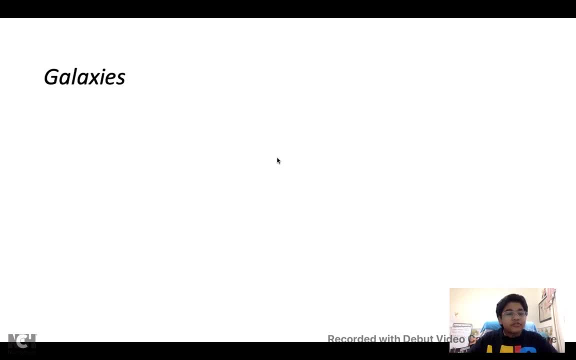 presentation now. so first thing we're talk about is galaxy, so you need to know what a galaxy is. so galaxy is a star, is stars and interstellar matter held together by gravity of a supermassive black hole in eighteen. in 2016, scientists estimated that they have 2 trillion. 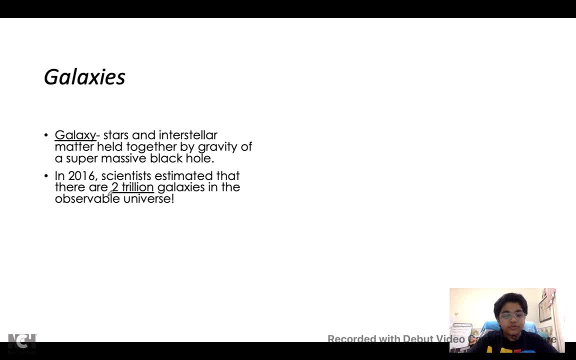 that there are two, two trillion galaxies in my, in the observable universe, and each galaxy contains hundreds of billions of stars. that's a lot of stars, three main shapes. here it comes up a spiral which we talked about in the last slide: elliptical, which I was gonna say, which I was unable to, and then irregular. so 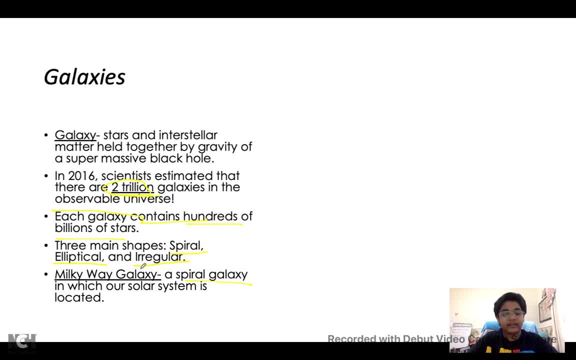 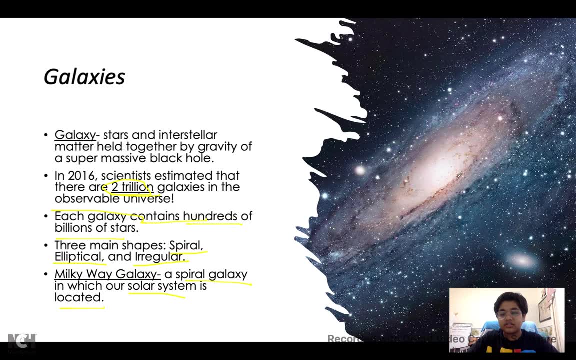 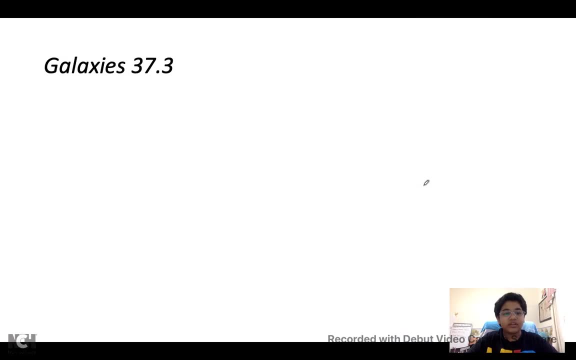 Milky Way galaxy is a spiral galaxy. we're taking this one in which our solar system is located. so this is the Milky Way galaxy. see how it's a spiral. yeah, so continuing on with today's galaxies unit that topic. okay, so thick interstellar dust gives it a Milky appearance, but also obscures the 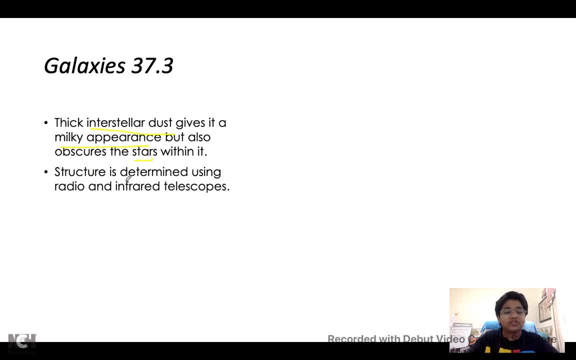 star system within it and structure is determined by using radio and ferret radio and in ferret telescopes and supermassive black hole, as in the center of your Milky Way galaxy. it takes hundred thousand light years in diameter. it's hundred thousand light years in diameter. so our revolution of our solar system takes 250. 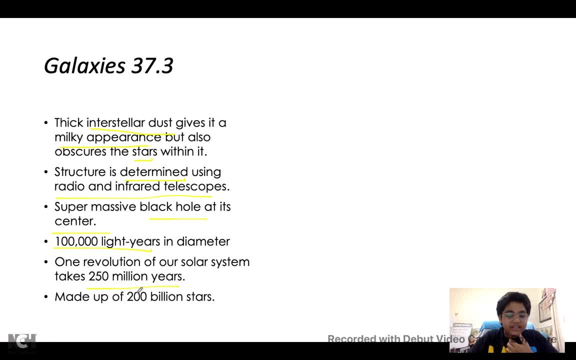 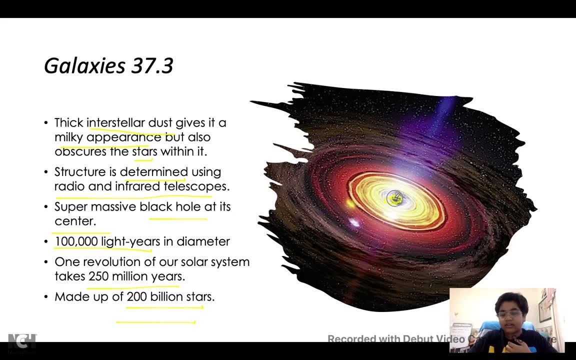 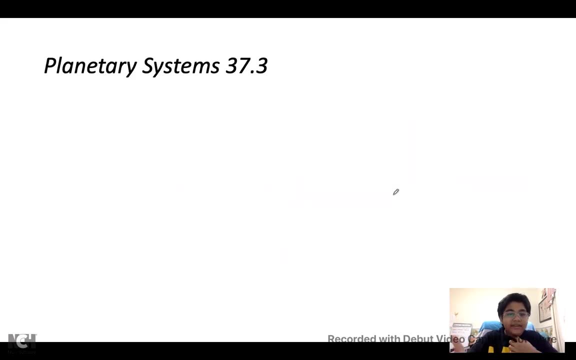 million years and it's made up of 200 billion stars. that is big. so here's a black hole. it's like right here in the middle of this spiral galaxy. yeah, so planetary systems now. so we're gonna learn about balance, planetary systems and galaxy, which is today. so planetary systems are system just made up a star. 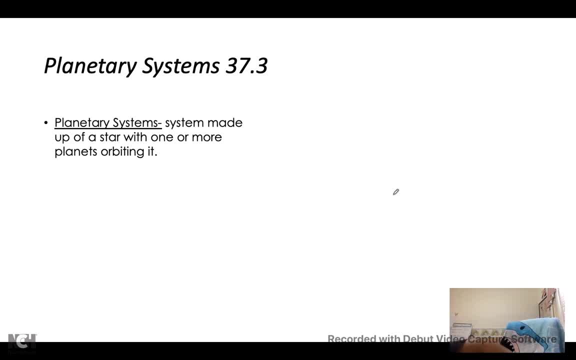 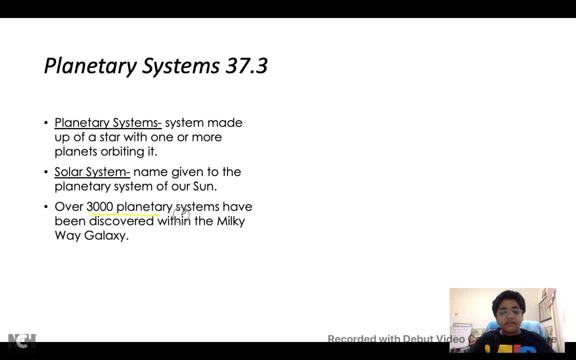 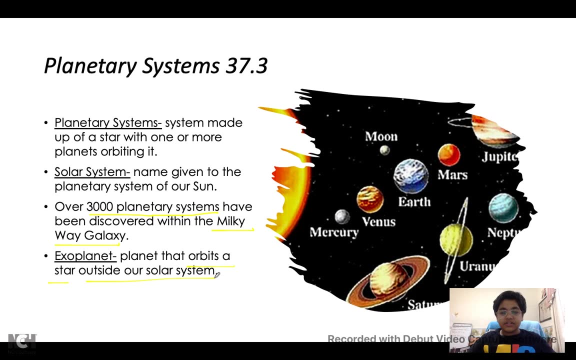 been discovered in the Milky Way, Milky Way galaxy. and then exoplanet is a planet that orbits, but the tanker through exoplanet because Goku brings the galaxy, because the link is a planet, then enter the galaxy. that has true every最後 anxiety. I'm gonna run into this next. 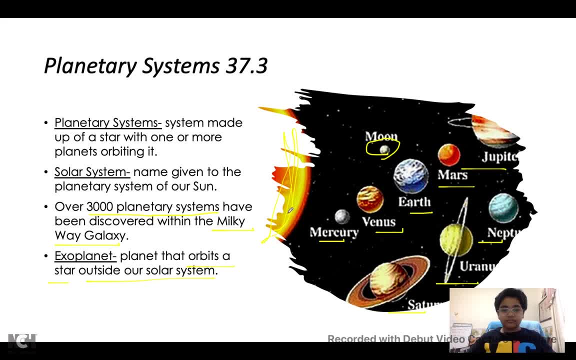 course, a star outside our solar system. so here is our plan вперy: Venus, Earth, which we live on, the moon, all the way over here, Mars, Jupiter, Saturn- you're a sinus- Uranus and Neptune- Pluto, if not there. and here's a sign, and yeah, so yeah. 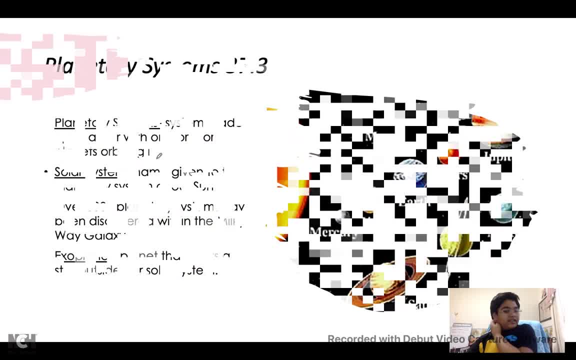 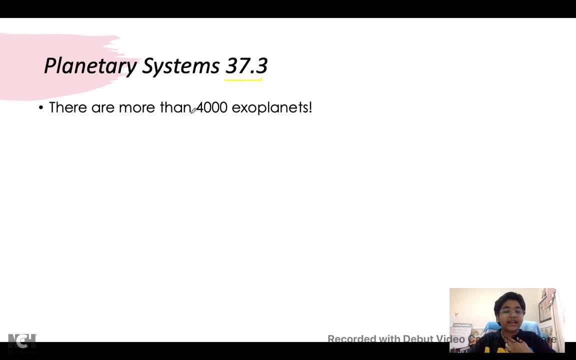 one or more planets orbit. okay, so planetary systems continued for today. um, there are more than 4 000 exoplanets- whoa, that is big. um, at least 55 of these uh exoplanets are in the habit habitable zone zone of their stars. habitable basically means they're able to live in on that. 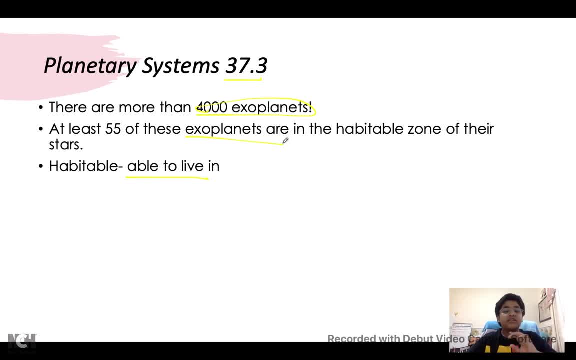 planet, five of the exo, 55 of the 55 of the exoplanets you're able to live on. and what did sinus look for? to determine a planet to support life, to look for, to determine if a planet can support life um one distance from star, which is like the goldilocks, is like oh, too hot, too cold. 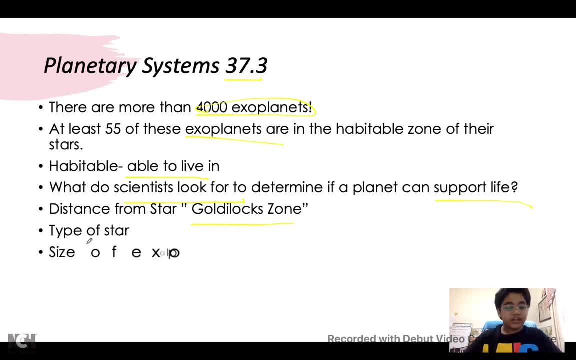 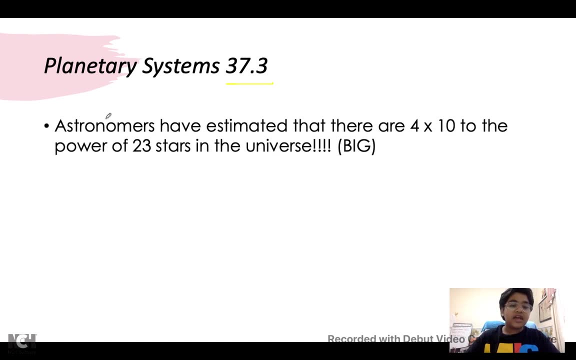 just the right one type of star, uh, the size of exoplanet and orbit, and the last one, atmosphere. so, yeah, so planetary systems continued for today. once again we have a lot of those. astronomers have estimated that there are four times ten to the power of 23 stars in the universe, which is 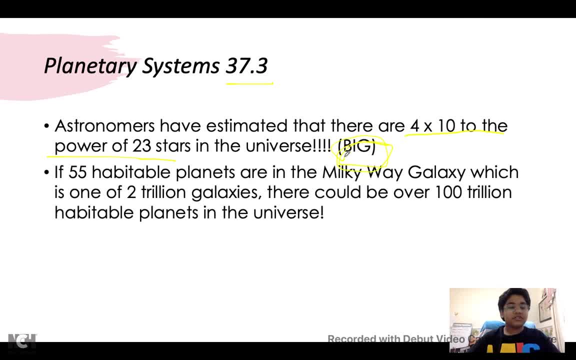 big. i don't even know how much it is in our uh uh powers of ten chart, but it's big, that's all i know. okay, if so, if five, if, oh my gosh, if 55 habitable planets are in the milky way galaxy, which of the one, two trillion galaxies? 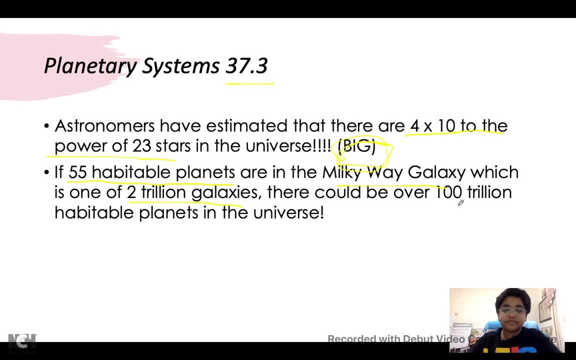 which is one of the two trillion galaxies there could, which is one of the two trillion galaxies there could be over 100 trillion habitable planets in the universe. big again, okay, the interstellar distance is an interstellar space and the interstellar masses are 15th and 16th million. 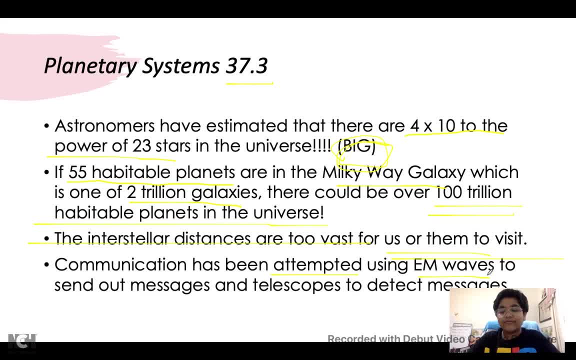 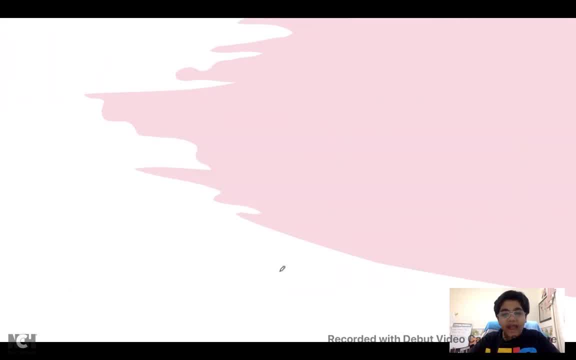 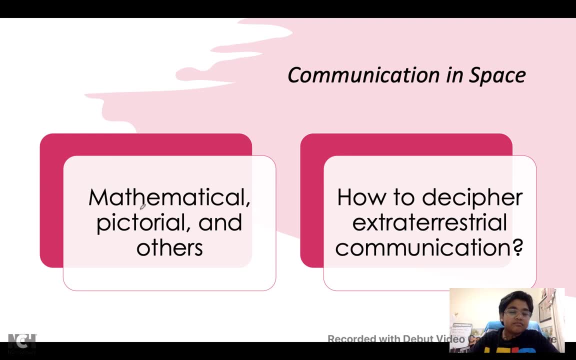 much like our solar system but, crossing some of the water libraries, we are able to get a, since there are two vast for us or them to visit, and communication has been attempted using em waves to send out messages and telescopes and detect messages. so now we're going to talk about communication in space, how they usually communicate. 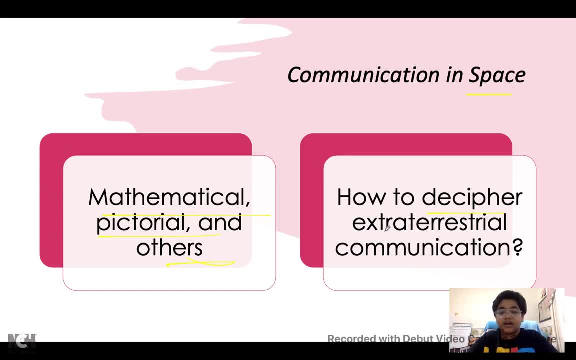 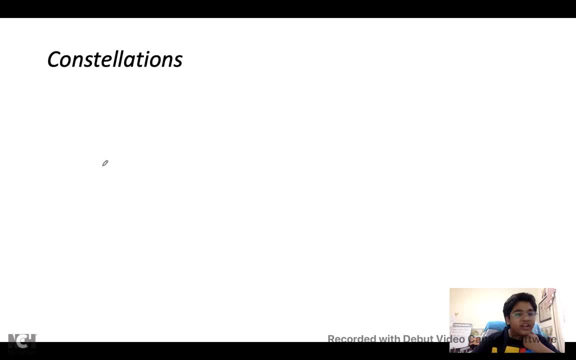 how to decipher, how they decipher in space a creature, extraterrestrial communication. okay, now we're going to talk about constellations. so constellation is an area in the sky in which a group of stars forms a pattern seen from the earth and representing the object, animal or person: the 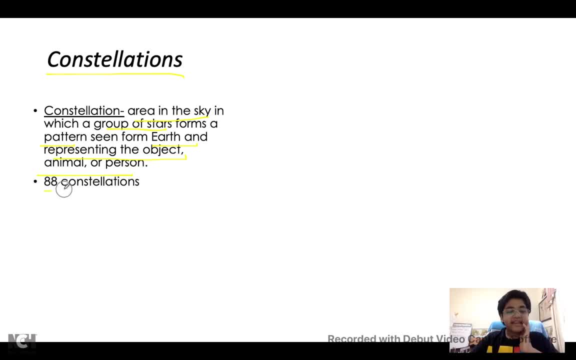 object: animal or person. there is 88 constellations in the world. okay, so are the constellations moving, or are we moving? so, parent motion? so as the earth rotates, this star- this includes our Sun- seem star, seem to move across the sky from east to west. actually, the stars are not moving, we are moving. 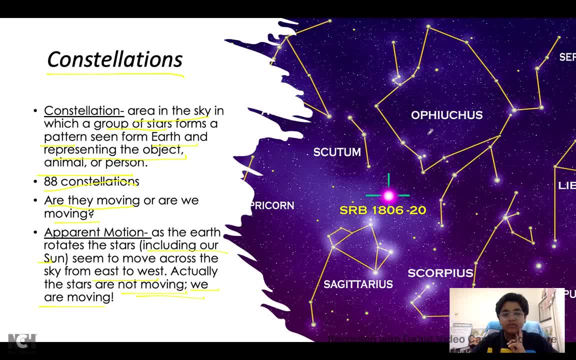 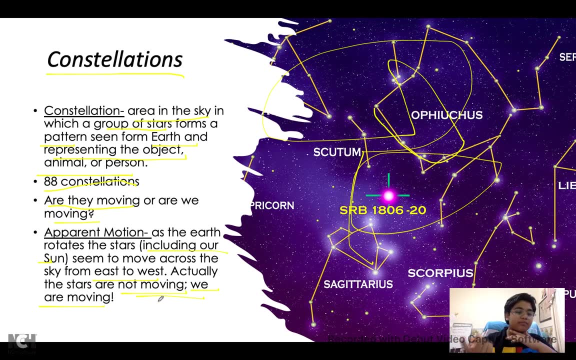 because the earth rotates, see. so here's what a constellation look like. if you're confused, oh, I don't know how to explain, but that's a constellation and this means we're- the stars are not actually moving. we're moving because, because our earth rotates on an axis points toward Polaris at 23.5 degrees in this. 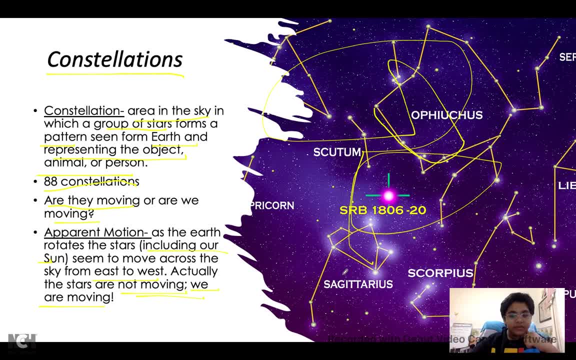 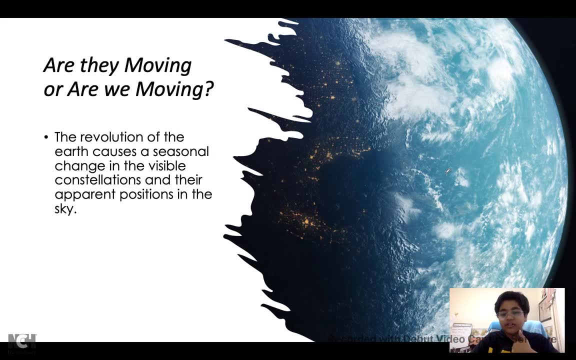 geo, but we're not moving. that's the same thing that happens to stars: they go away at morning and then they come back at night- today night, because earth is rotating. okay, uh, are they moving or are we moving? so I just showed a picture here of the Earth, like: are they moving or we moving? is the earth moving or the constellations?